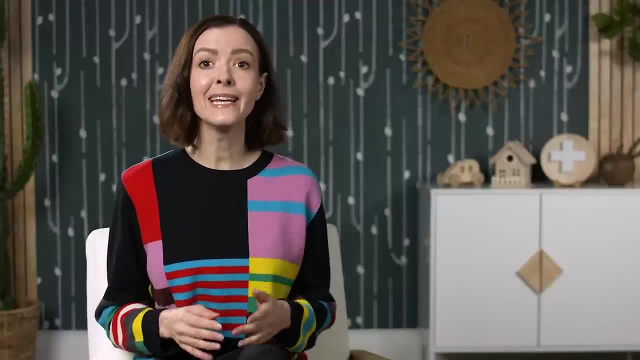 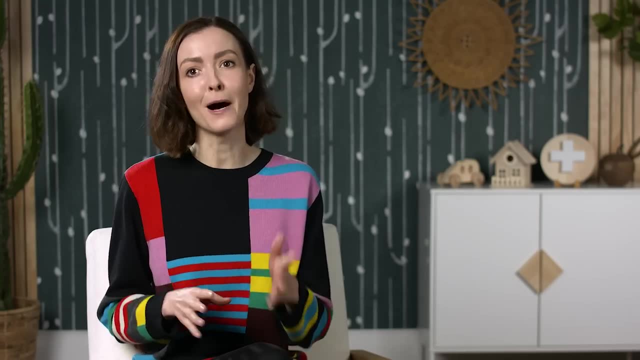 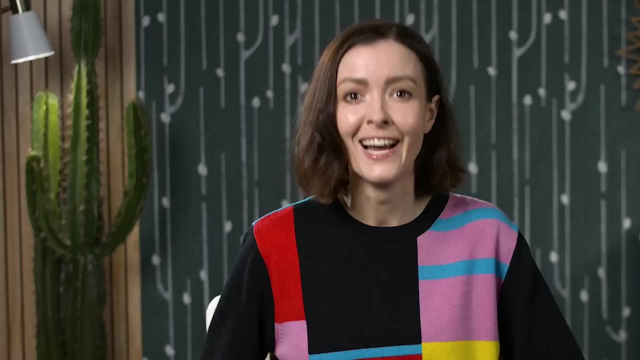 But no matter which kind of epidemic we're studying, we need epidemiology to help us do it. Epidemiology is basically where all the science-y stuff happens in public health. It uses microscopes, data, math and pie. Don't worry, we'll get to that. 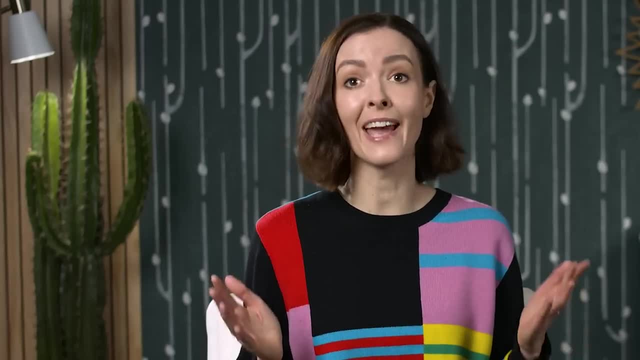 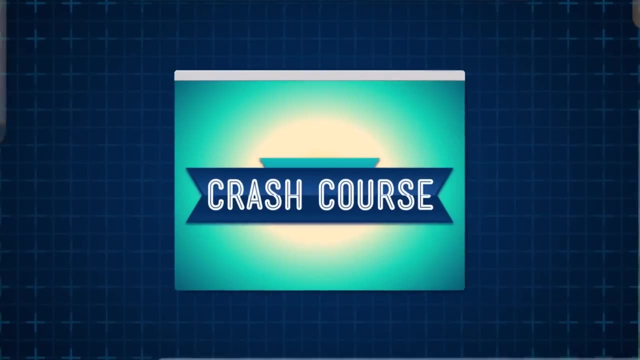 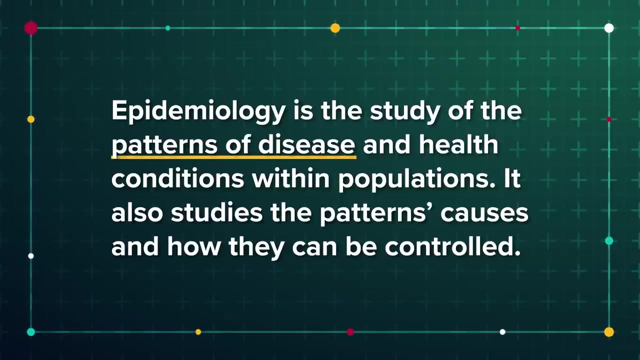 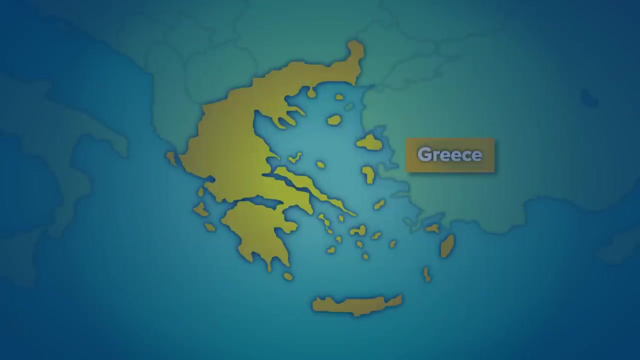 Hi, I'm Vanessa Hill and this is Crash Course. Public Health Epidemiology is the study of the patterns of disease and health conditions within populations. It also studies the patterns' causes and how they can be controlled. Much like Democracy and the Mamma Mia film franchise, we can at least partially give. 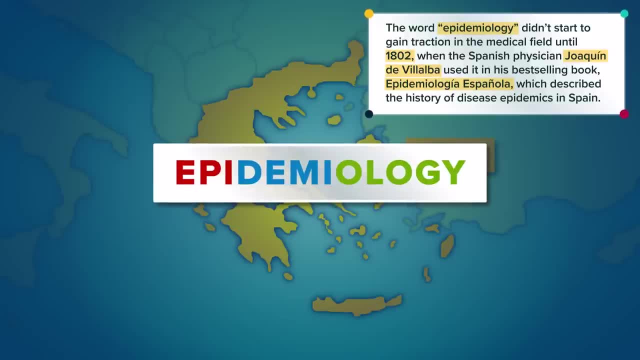 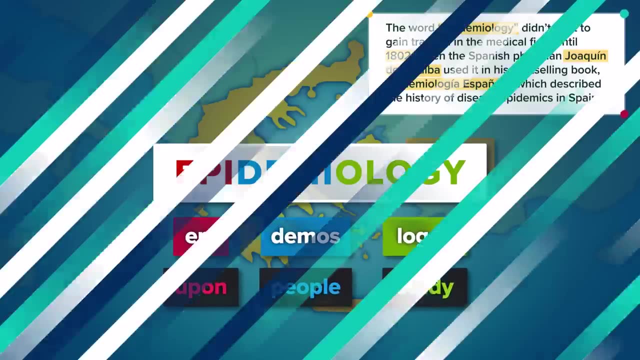 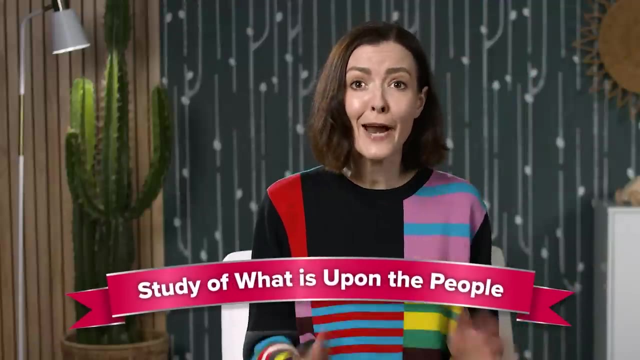 credit for the word Epidemiology to the Greeks. It comes from the three Greek words epi, demos and logos, which mean upon people and study. So epidemiology is literally the study of what is upon the people, which is kind of a terrifyingly broad field. 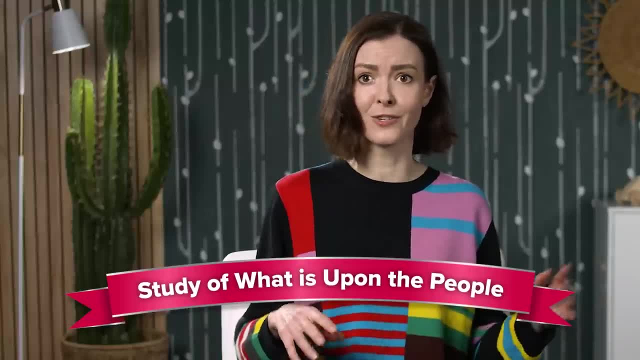 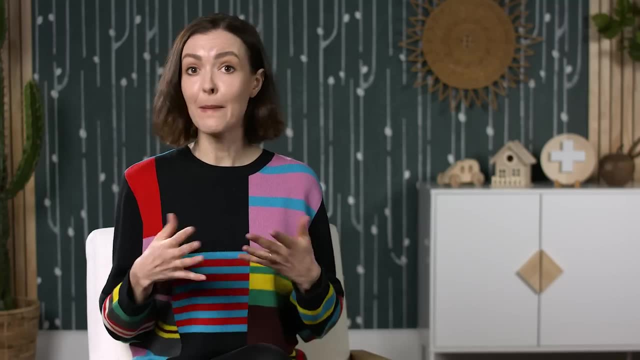 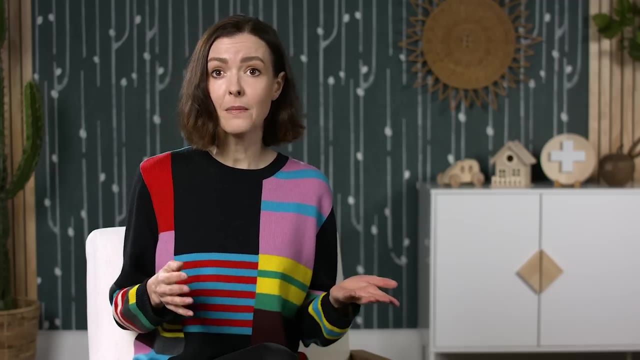 the people could describe anything from climate change to whatever Hank Green is plugging on TikTok today. be sure to check out the link in his bio. But anyway, to specify, an epidemiologist or someone who studies epidemiology wants to know who gets what diseases, where they get them and when. 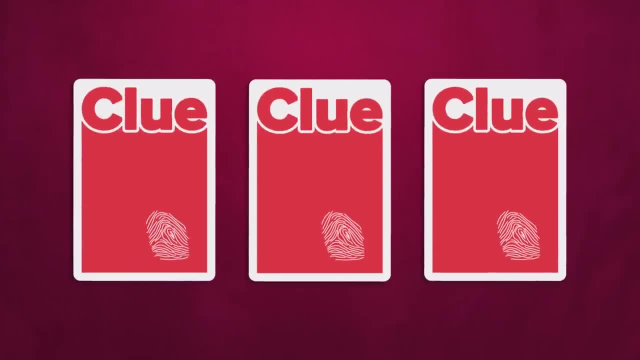 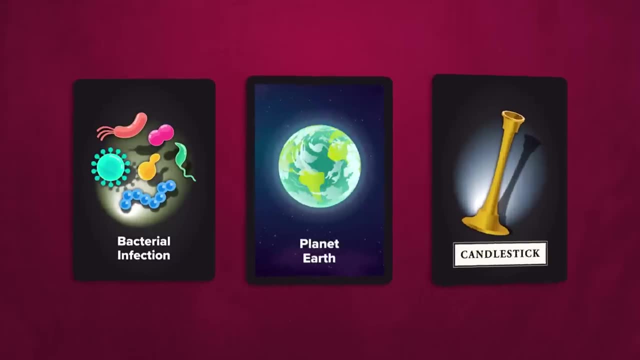 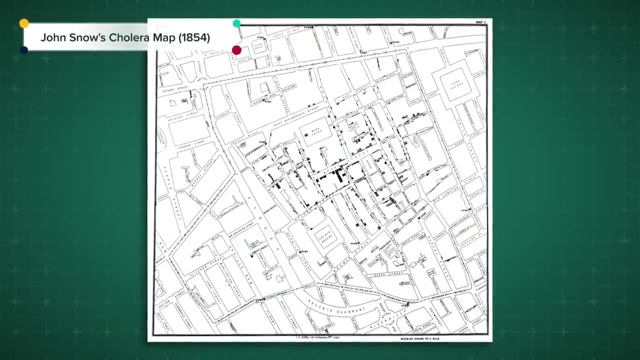 Epidemiologists are kind of like detectives in a massive game of Clue or Cluedo, except instead of Professor Plum in the ballroom with the candlestick. it's more like a bacterial infection on planet Earth that threatens literally everyone. The word and the actual practice of epidemiology didn't gain traction until the 19th century. 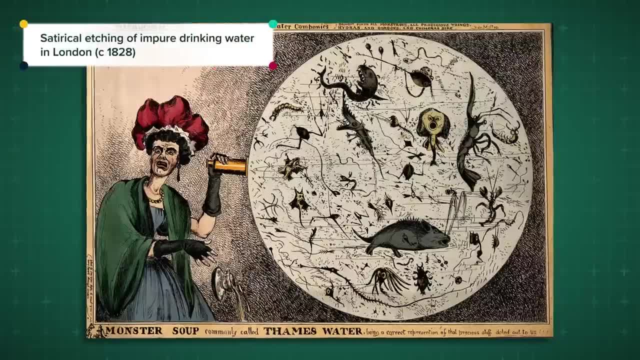 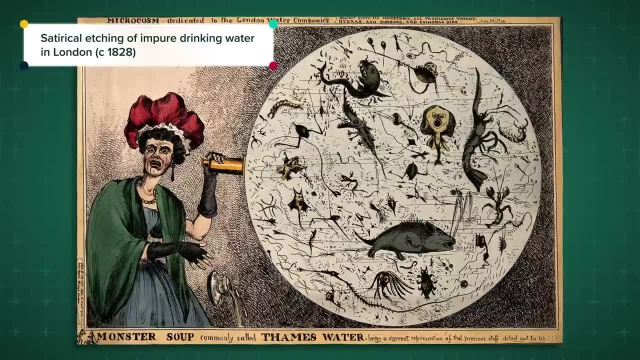 when it mostly concerned infectious diseases. These are health conditions caused by organisms like viruses, bacteria and parasites, which are spread between people or picked up from the environment or animals. But today we understand why. We understand, why We understand epidemiology more broadly. 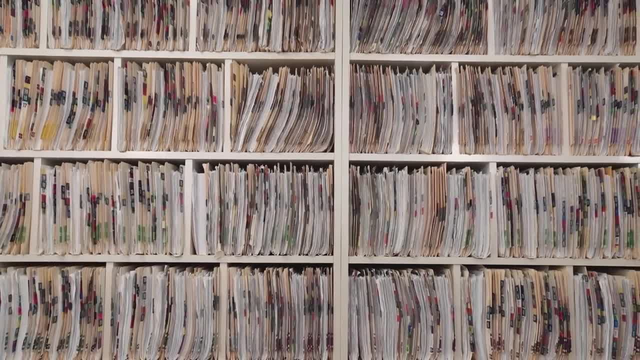 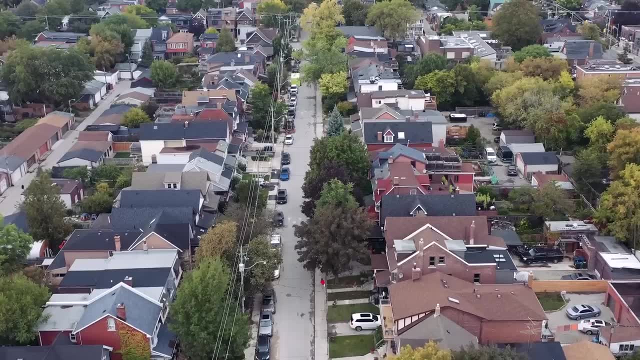 This is partly because we also understand health more broadly And, as we saw in our episodes on the determinants of health, our health is affected by more than just germs. It's also impacted by our neighborhoods, schools and society in general. 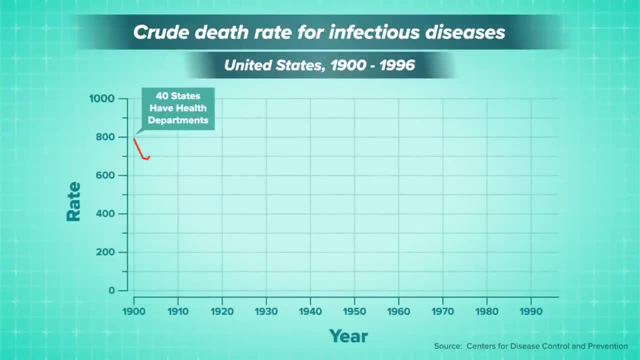 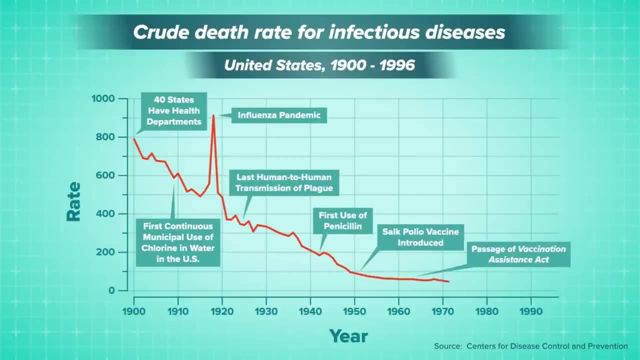 But we also understand epidemiology differently, because, at least in high-income countries, causes of death have changed, as advances in medicine and public health have meant fewer deaths from infectious diseases. in these places, Non-infectious, also known as non-communicable causes of death have become a bigger area. 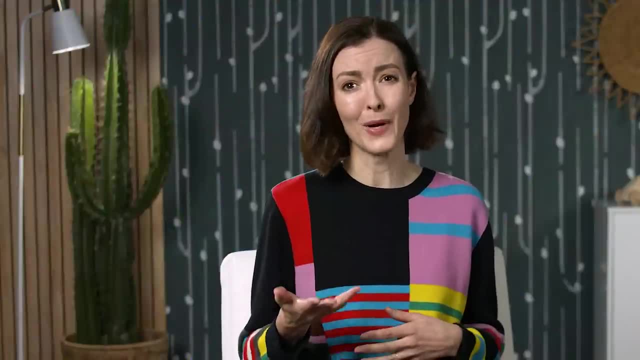 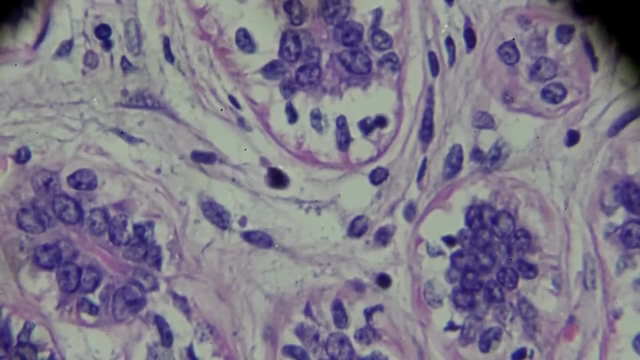 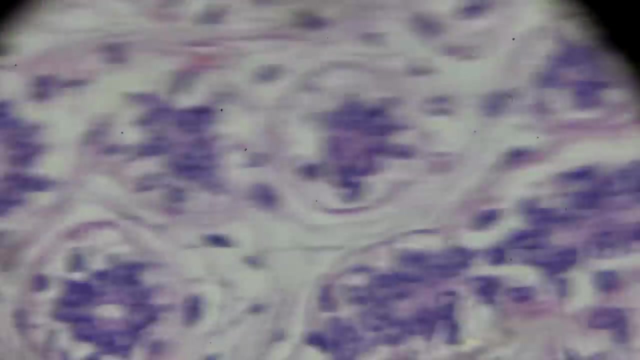 of focus. We know that's pretty unfair for lower-income countries. We'll talk about that in episode 9, when we focus on global health. So today many epidemiologists put more emphasis on studies of non-communicable diseases like cancer, heart disease and diabetes. 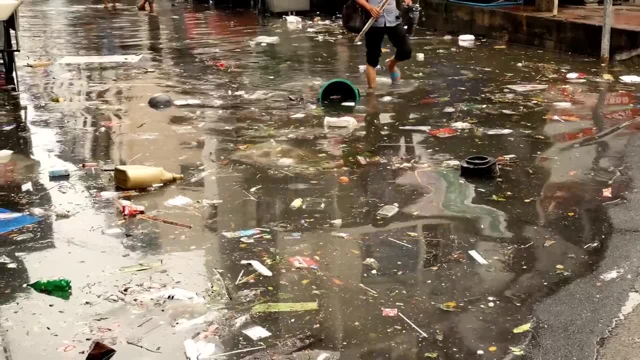 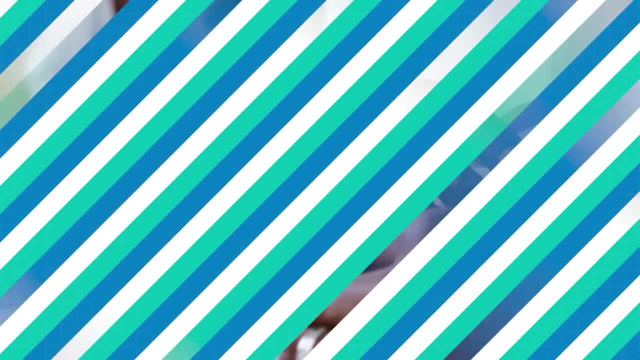 Environmental factors like air pollution are also important, And even the health impacts of natural disasters. They also examine the determinants of health and the inequities in who gets sick. That's also what we'll be focusing on today, though, over at Crash Course Outbreak. 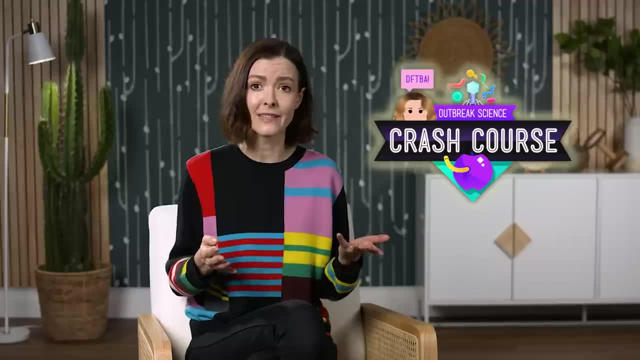 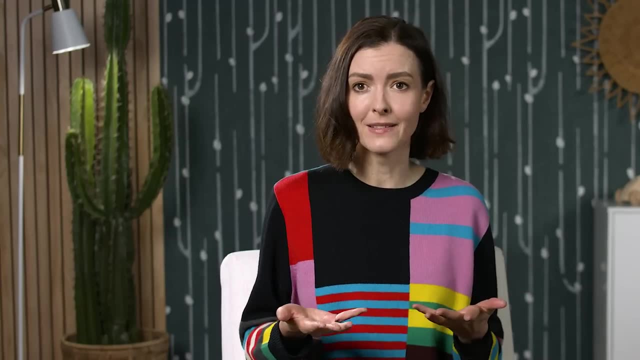 Science. we spend plenty of time talking about infectious diseases, including how public health tackles them. We know, with any big mystery, it's not enough to know that something happened. We want a motive. So, as epidemiologists solving a health mystery, we want a motive. 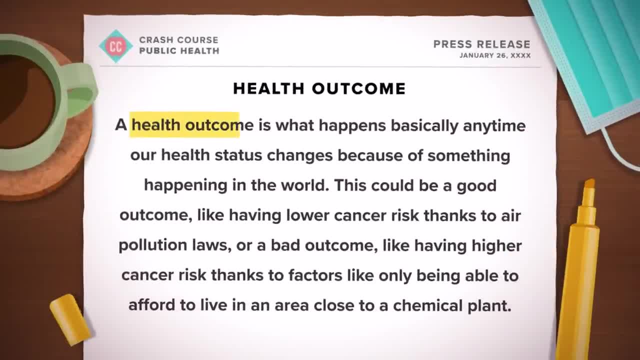 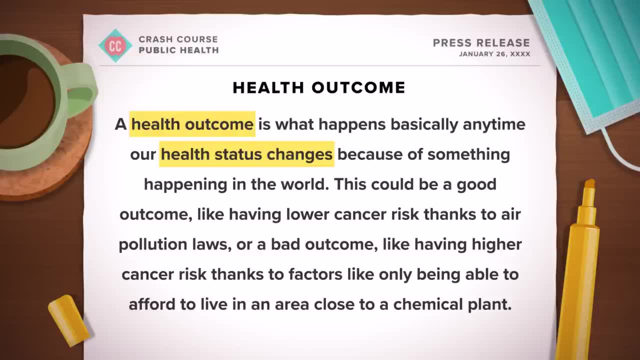 We want a cause for that health outcome. A health outcome is what happens basically any time our health status changes because of well something happening in the world. This could be a good outcome, like having lower cancer risk thanks to air pollution laws. 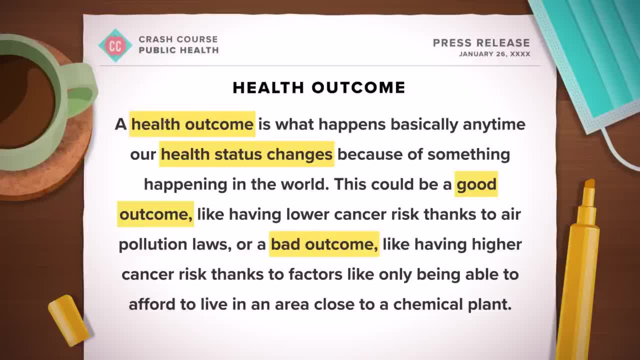 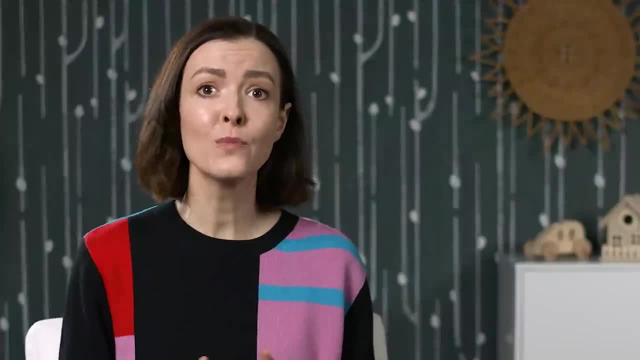 Or a bad outcome, like having higher cancer risk thanks to factors like only being able to afford to live in an area close to a chemical plant. Epidemiologists begin with a hypothesis about why a health outcome can be a cause for a health outcome, Why a health outcome is spreading or occurring in the first place. 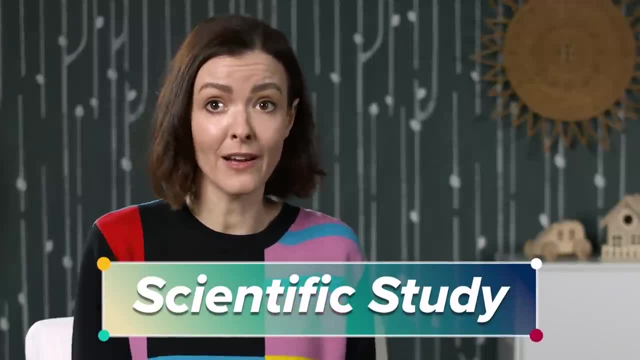 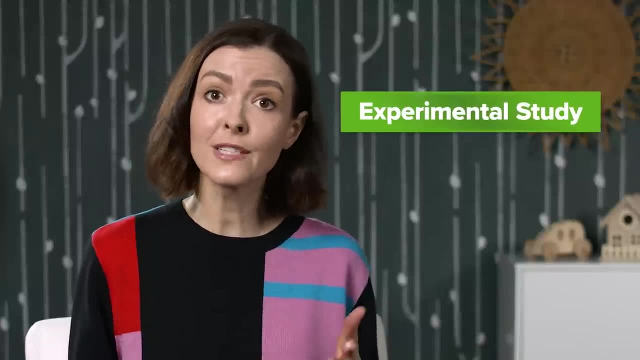 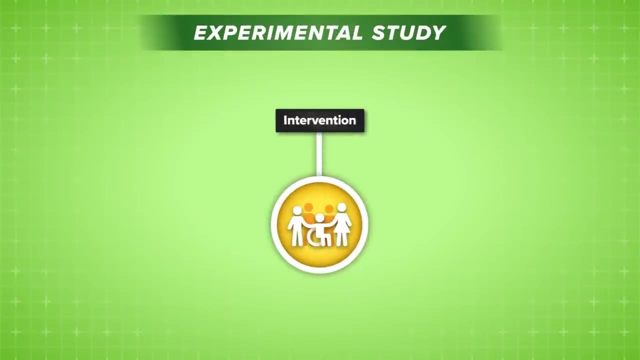 Then they conduct a scientific study to evaluate their hypothesis. In general, there are two kinds of epidemiological studies that we'll focus on here: experimental studies and observational studies. In an experimental study, investigators expose participants to some kind of intervention or treatment to see how it affects their health. 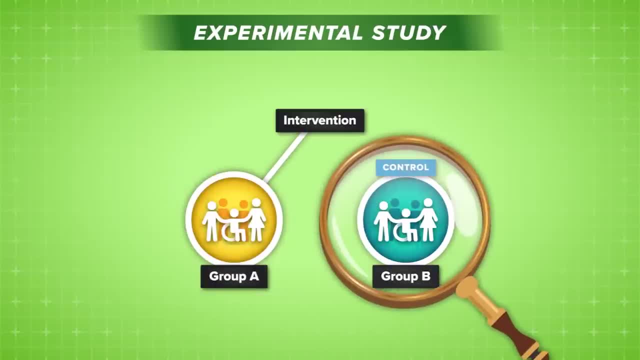 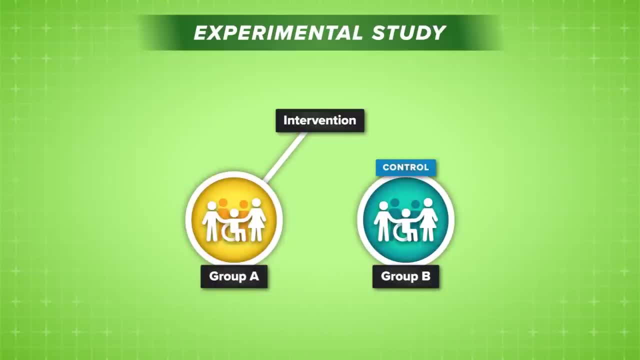 Then they compare the outcomes to a control group that isn't exposed to the intervention. Then they compare the outcomes to a control group that isn't exposed to the intervention. Now it's pretty unethical to expose a group of people to something that could harm. 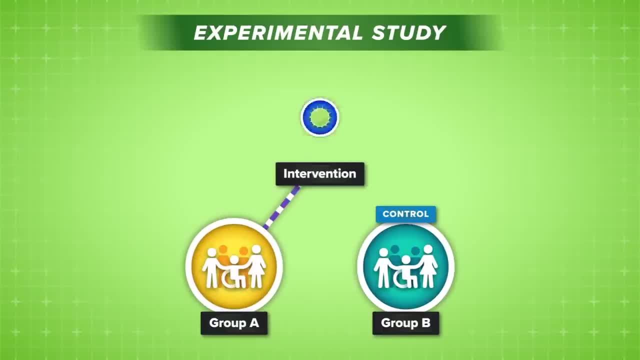 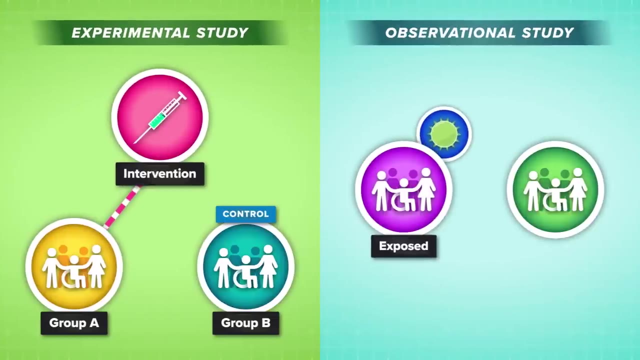 their health, So experimental studies tend to introduce positive interventions. This might include something like a new vaccine, as opposed to a negative intervention like a virus. In observational studies, epidemiologists observe a population that is already exposed to a particular treatment or risk factor. They observe the population that is already exposed to a particular treatment or risk factor. They compare their health to a non-exposed group. This is how we go about understanding the effects of things we don't want to intentionally expose people to, like viruses. 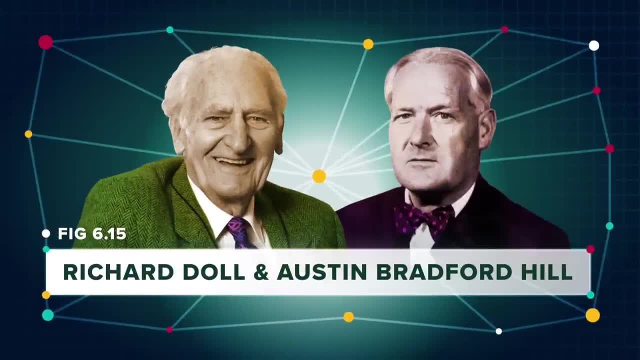 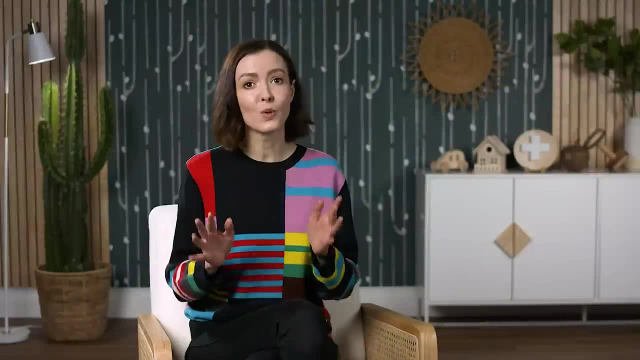 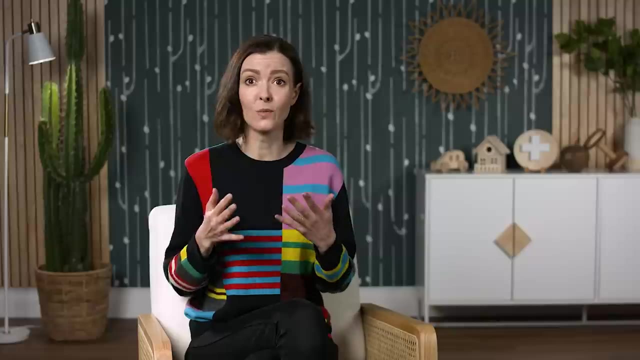 One famous observational study was conducted by a pair of British epidemiologists, Richard Dull and Austen Bradford Hill, no relation to me. In the mid-20th century it was widely known that lung cancer rates were on the rise, but there wasn't a scientific consensus on why. 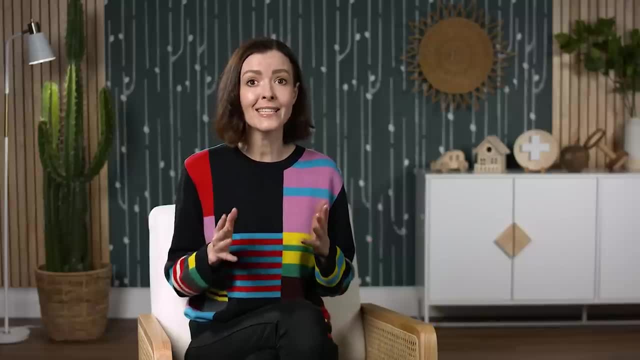 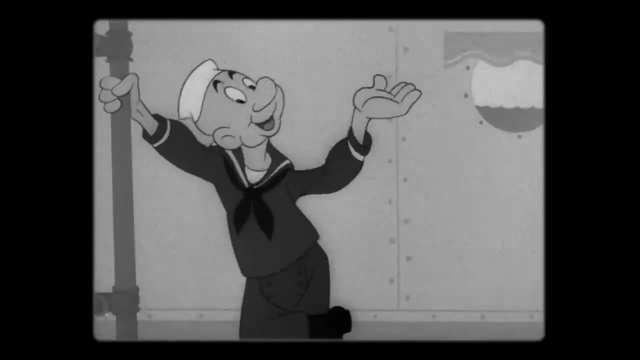 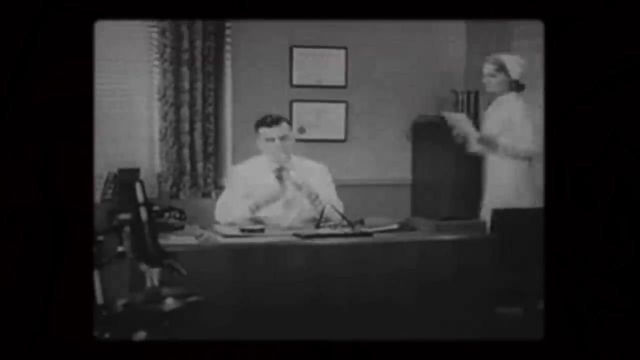 In 1951, Dole and Bradford Hill began testing a hypothesis for this increase – smoking. The idea that smoking can lead to certain kinds of cancer is pretty common knowledge today, But while some research pointed to an association between smoking and cancer, there wasn't. 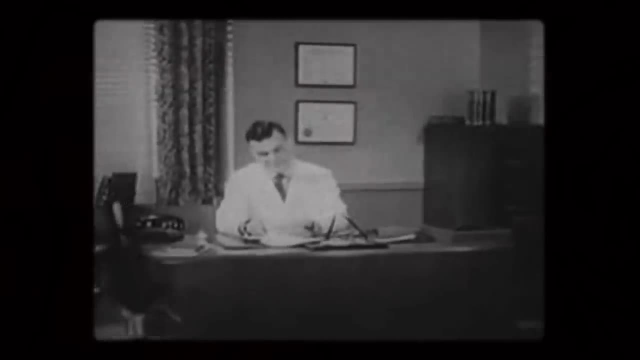 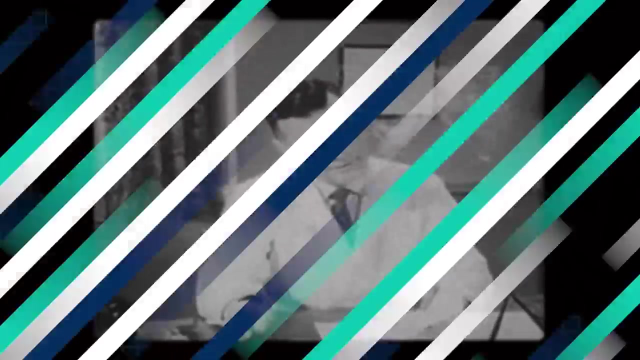 enough evidence to confirm that one event caused the other. In fact, smoking wasn't even formally recognized as a public health issue in the United States at the time. They sent out surveys to almost 60,000 British doctors asking about their smoking status. 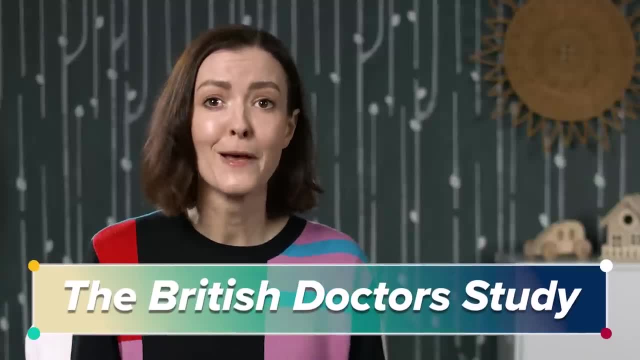 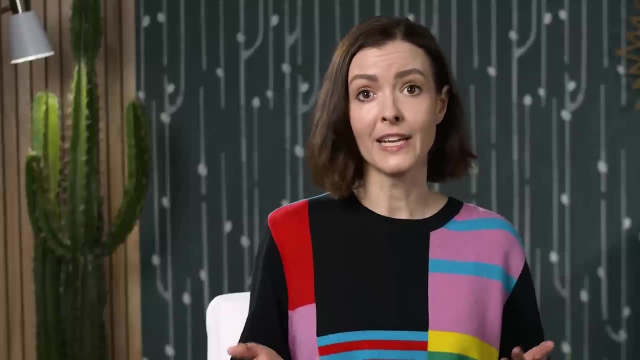 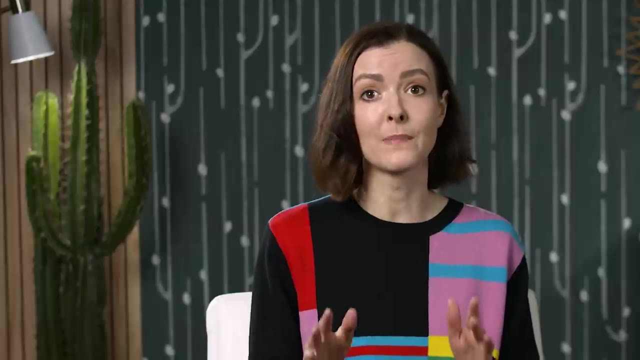 in a study that experts have so ingeniously dubbed the British Doctors' Study, And after getting over 40,000 responses, Dole and Bradford Hill found a strong association between heavy smoking and lung cancer, And repeated follow-up studies of the same doctors over the next 50 years confirmed the 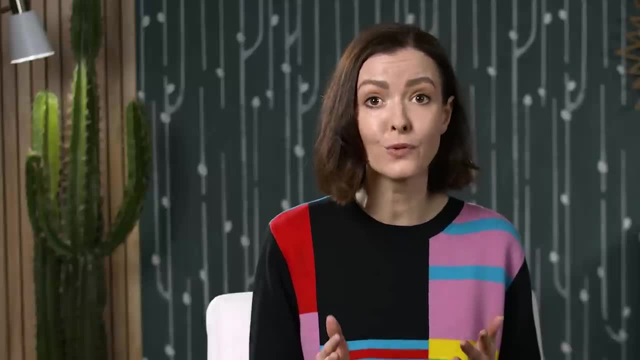 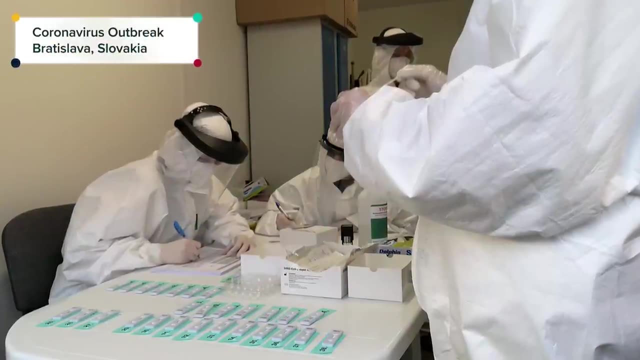 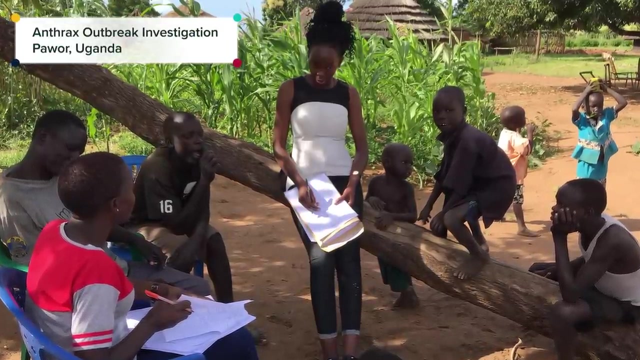 originally reported relationship of smoking and cancer. This led to several different kinds of cancers, including lung and mouth cancer. Unfortunately, when it comes to identifying the cause of a particular health effect, we don't always have the luxury of 50 years of research and 40,000 British doctors on. 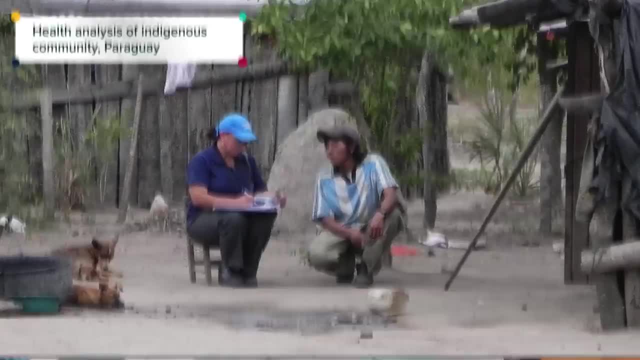 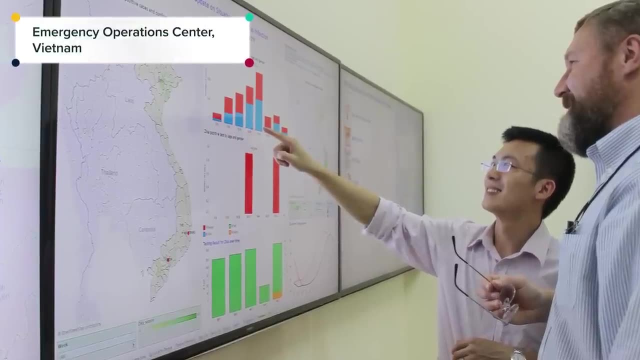 hand, Epidemiologists often have to work quickly to assess and respond to a health emergency, Regardless of the timeline involved. interpreting data is where epidemiology gets tricky, because data on its own don't tell the story, And that's why we're here today. 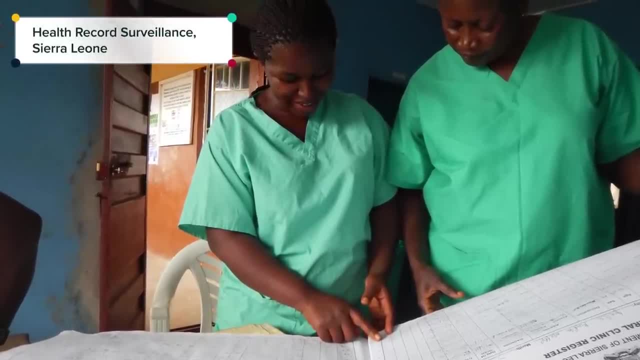 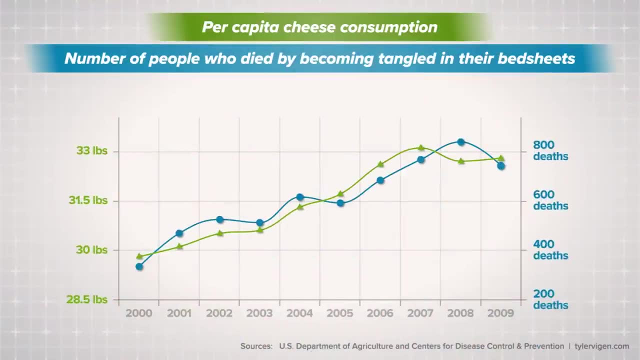 For data to be useful, they need to be interpreted by people, And data aren't always straightforward. Like data have shown that there is a near-perfect relationship between a population's level of cheese consumption and the number of people in that population who die from getting tangled. 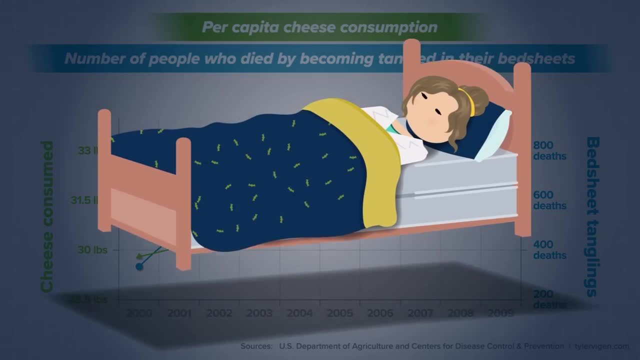 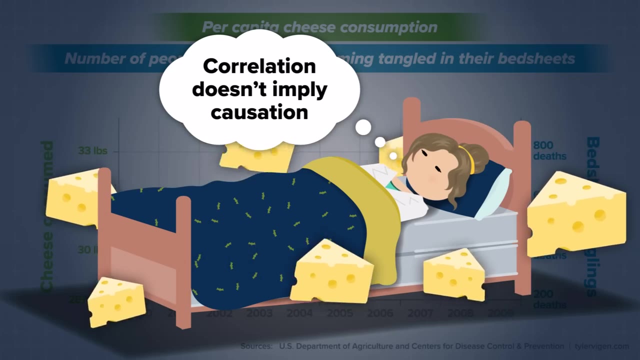 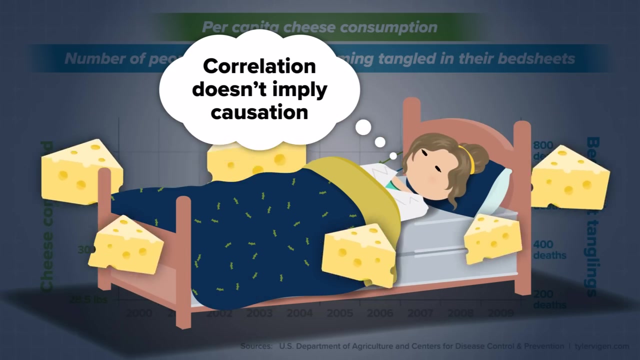 in their bedsheets. This is a very strange but true example of a cliché that scientists have been muttering in their sleep for centuries. Correlation doesn't imply causation, Or put another way, just because two things seem related doesn't mean that one caused. 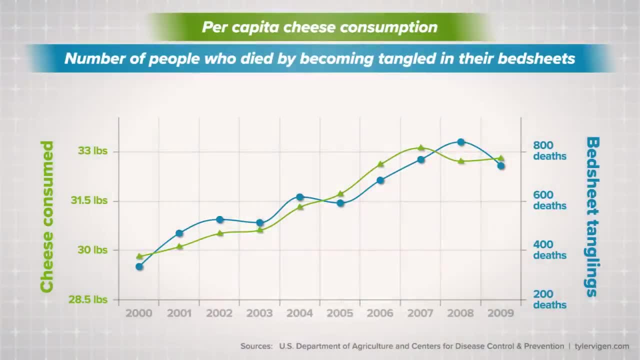 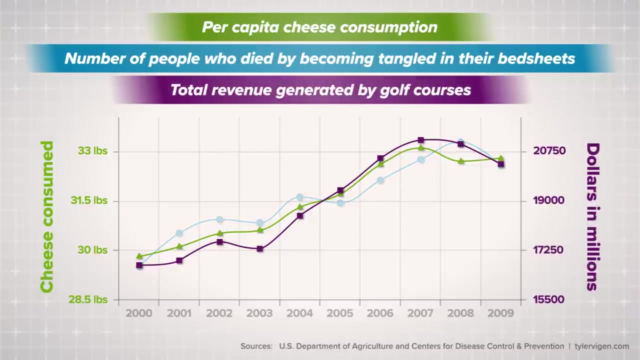 the other. So, while the data appear to say that cheese consumption and bedsheet murder both increase at the same time, we need someone like an epidemiologist to examine and interpret the data, to tell us whether that actually means anything or if cheese consumption just happens. 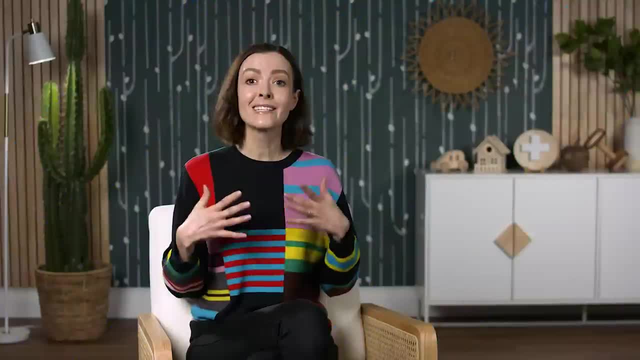 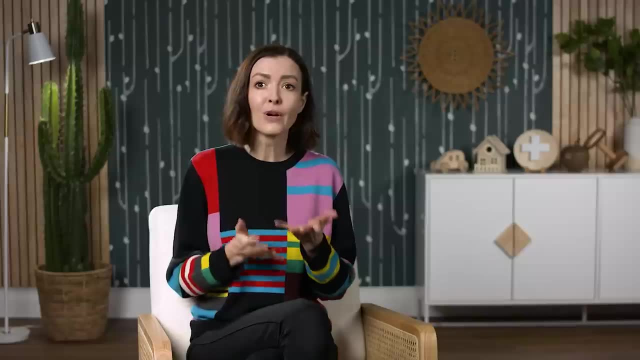 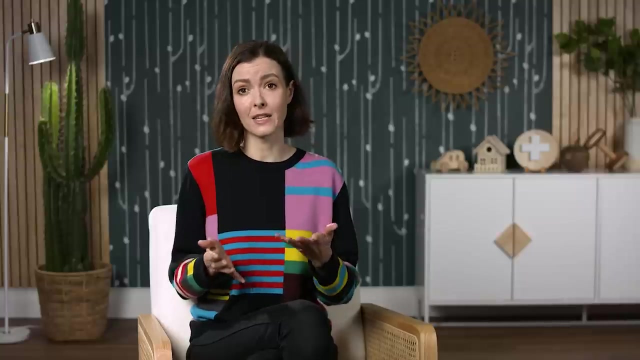 at a similar rate to a lung disease of other things. To successfully interpret data, epidemiologists need to rely on several pieces of evidence. Like while the British Doctors' Study was one of the first population-level studies that linked smoking to lung cancer. this wasn't a new idea at the time, As Dole and Bradford Hill. 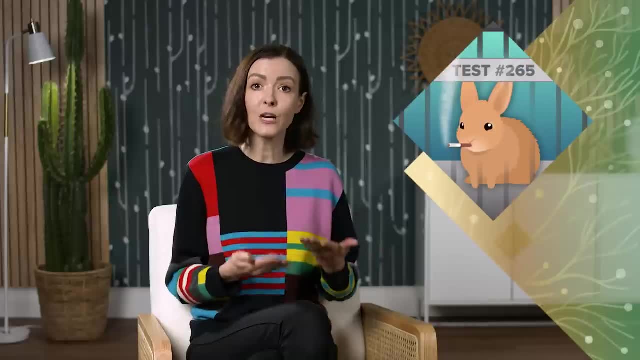 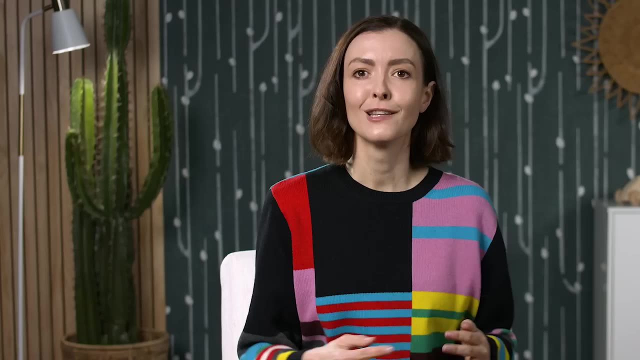 conducted their studies. they were following in the footsteps of animal-based studies and chemical analyses of tobacco that had been happening as far back as the 1900s. Like a lot of science, their conclusion wasn't the product of two dudes doing a thing. It took. 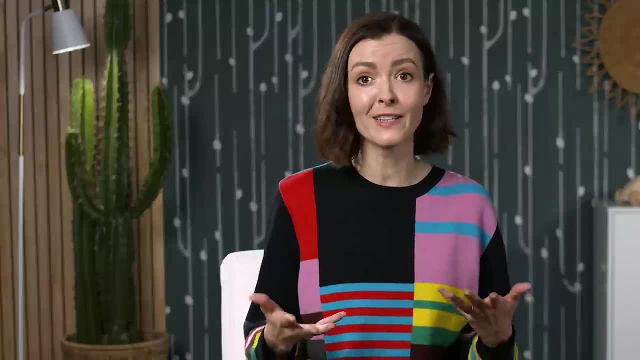 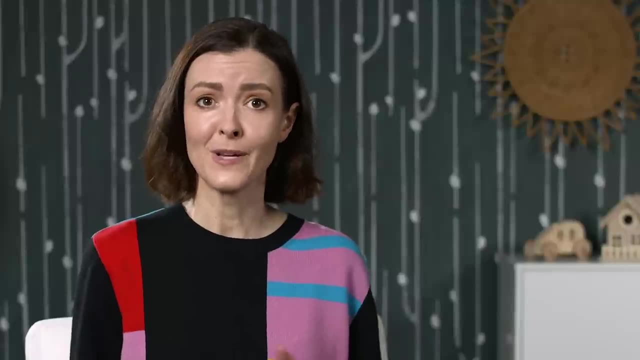 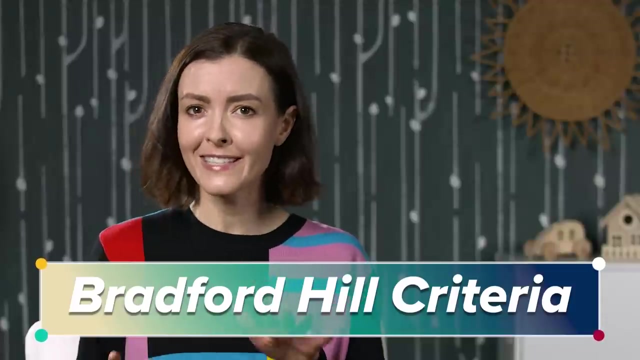 decades of collaboration between a bunch of people in different disciplines, each following their own unique path of evidence to the same conclusion. One useful tool epidemiologists use to understand the cause of an observed effect is the Bradford Hill Criteria. And yes, that's the same Bradford Hill from the British Doctors' Study Small world. 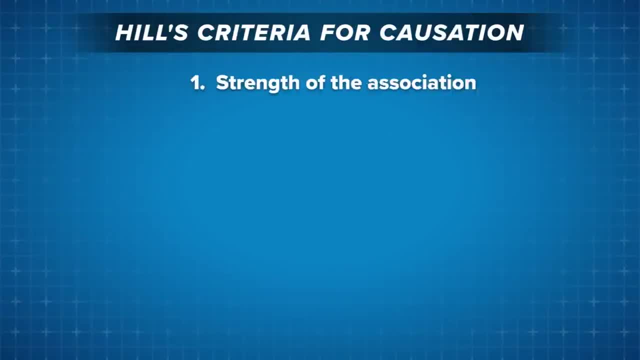 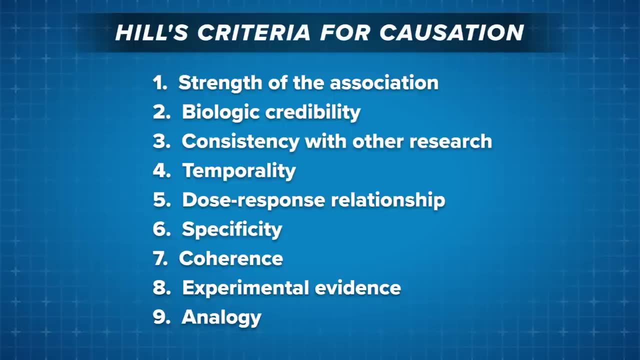 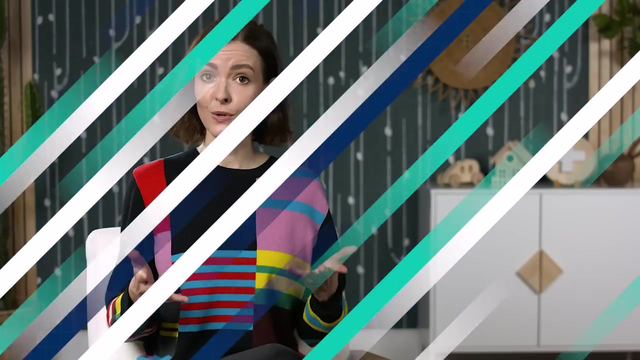 While we won't get into all of them here, Bradford Hill proposed nine principles for establishing evidence of a causal relationship between a presumed cause and an observed effect, Like whether the effect happened after the cause or if the effect could be reproduced. Another tool epidemiologists use to better understand the sometimes 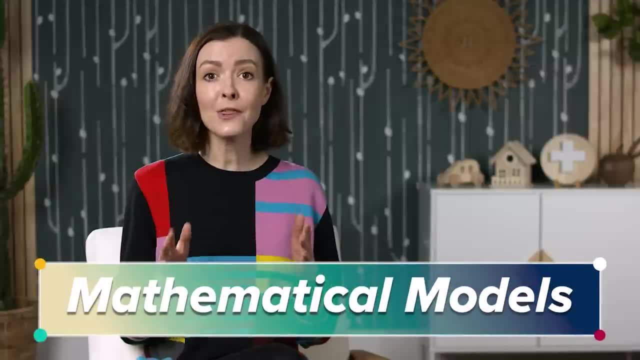 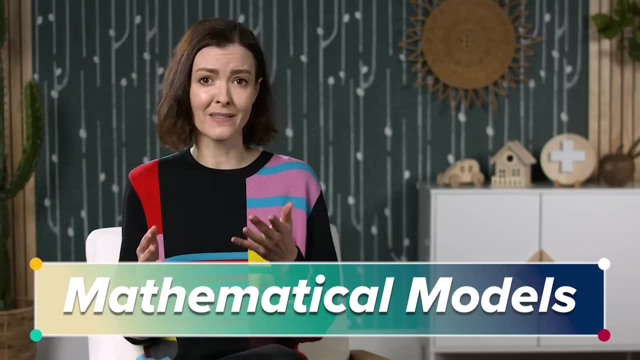 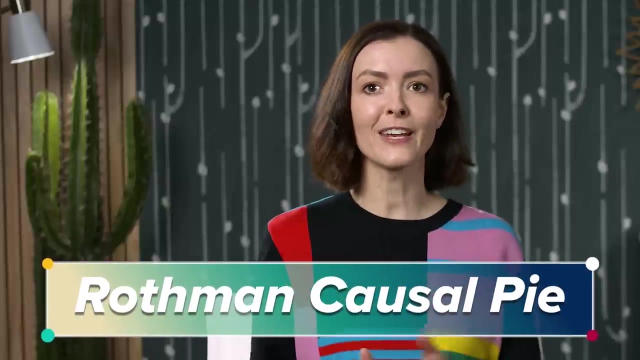 messy relationship between cause and effect is mathematical models. These models tell epidemiologists which variables are worth paying attention to and which ones aren't, Which brings us at long last to pie. The Rothman Causal Pie is a model that helps epidemiologists explain how individual risk 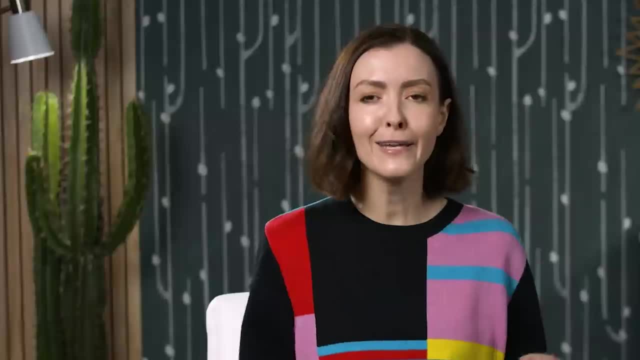 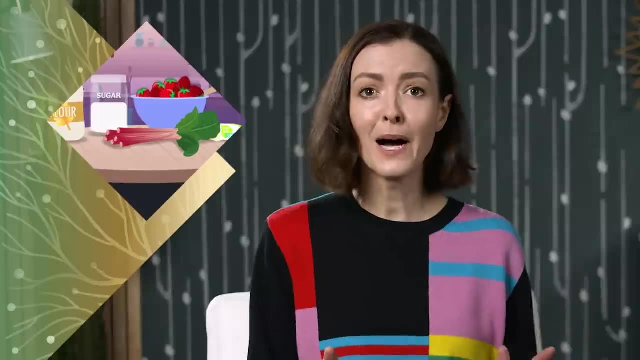 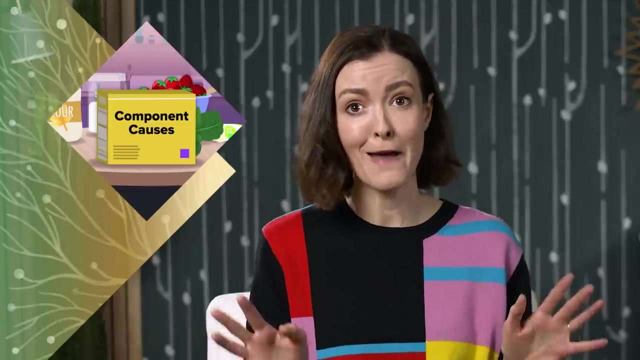 factors contribute to a disease And, like any good pie, a causal pie needs a few different ingredients. Except, instead of sugar and rhubarb, this pie is made up of component causes, which probably settles the debate about the worst pie flavor ever. Component causes are basically the: 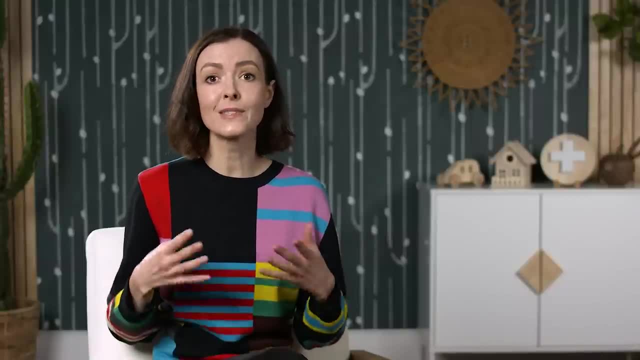 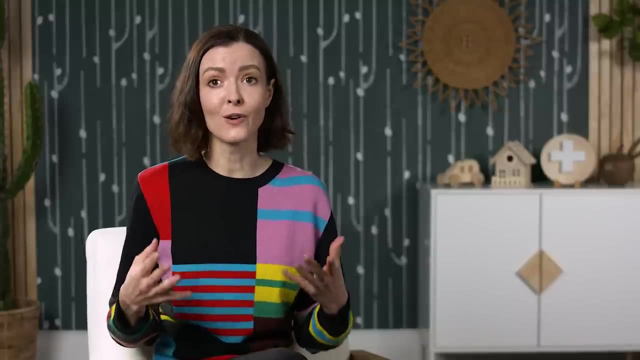 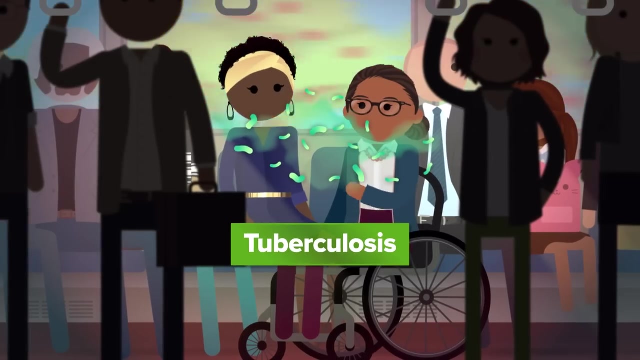 different risk factors that work together to produce a certain health effect. pie, If we have enough cause, slices to form a whole pie. we have a sufficient cause, which means the health condition goes into effect. Let's go to the Thought Bubble. Let's consider tuberculosis or TB. 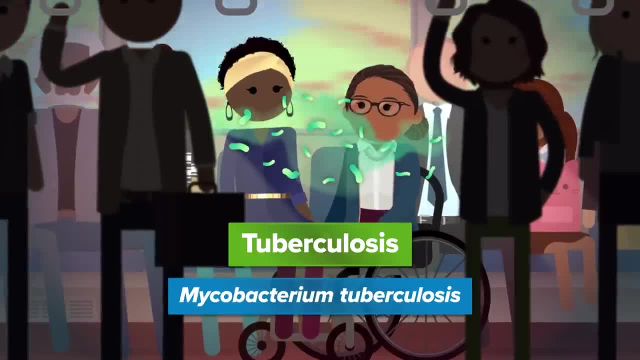 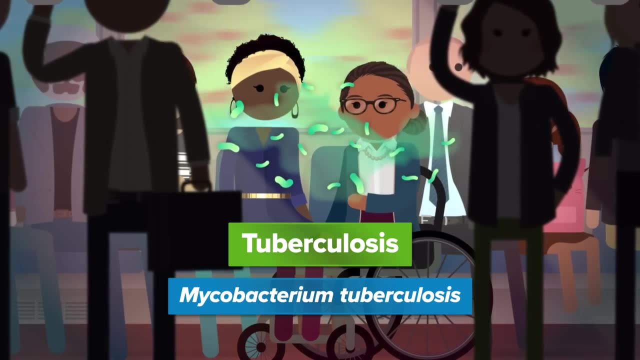 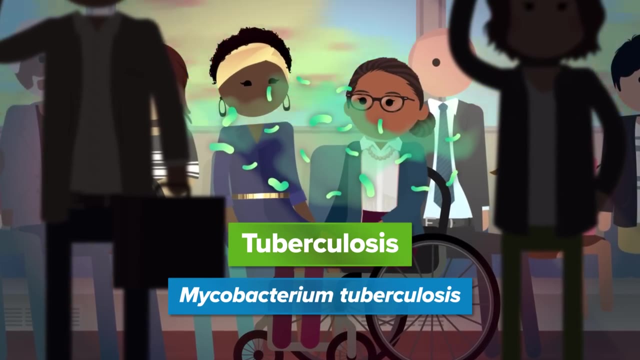 a highly infectious disease caused by the bacteria Mycobacterium tuberculosis. Because TB is an airborne pathogen, it's generally spread through a pretty basic human action – breathing, And when you have too many people breathing in the same space and one of them is sick, there's a higher risk for transmission. 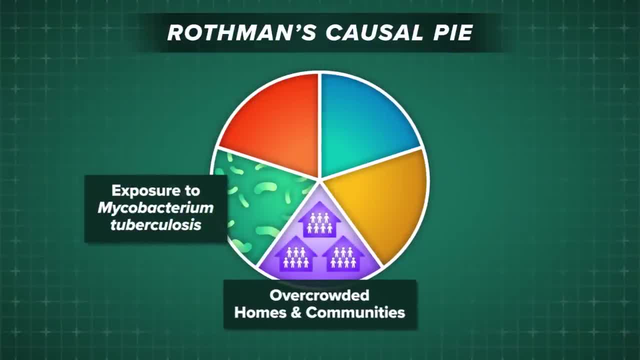 So we might consider overcrowded homes and communities to be one slice of the causal pie. Similarly, buildings with poor ventilation will be worse at getting rid of airborne bacteria, making poor ventilation another notable component cause. Another component of our pie is having a weakened or compromised 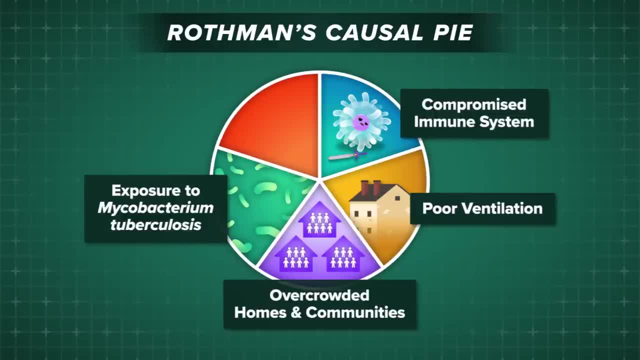 immune system. Basically, if our body isn't as good at fighting off disease, it's also more likely to get sick from exposure to the bacterium. Similarly, lack of access to a tuberculosis vaccine means our bodies will be more likely to contract the disease. so that's also a pretty big part of the causal pie. 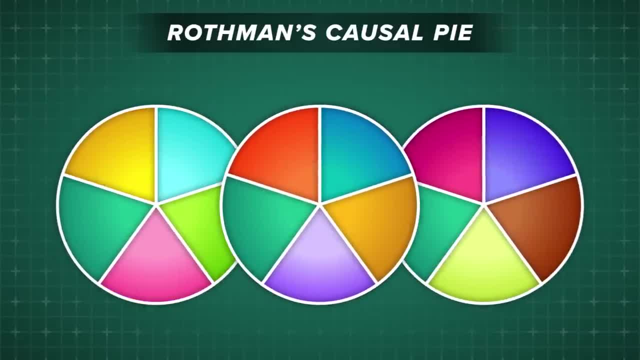 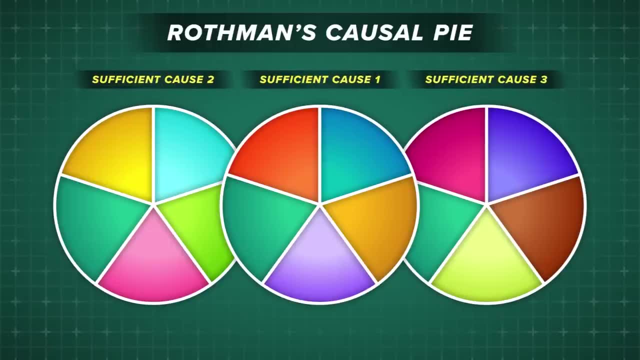 Just like how everyone cuts a pie differently, everyone will have a different combination of component causes that combine to produce a sufficient cause for TB. But one slice that's in every causal tuberculosis pie is exposure to mycobacterium tuberculosis. This is because TB can't like spontaneously generate in our bodies. It needs a source. 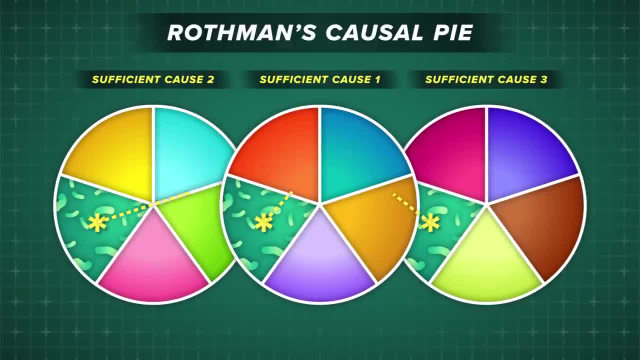 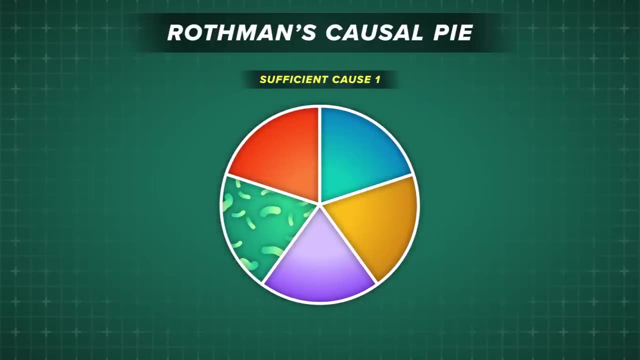 This is why exposure to mycobacterium tuberculosis is a necessary condition of TB, Even if all the other risk factors of the pie are in place. mycobacterium tuberculosis is needed to activate the disease Now, while the presence of each individual risk factor increases the likelihood of TB. 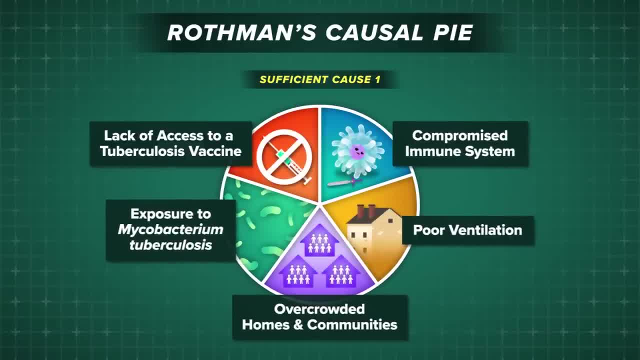 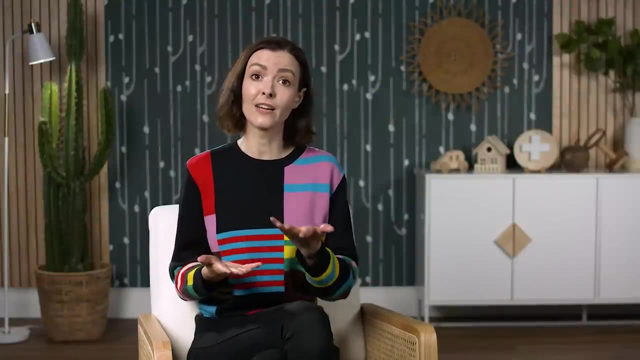 it doesn't guarantee it. But if we fill up our causal pie with a combination of components that produces a sufficient cause, we get our health outcome. tuberculosis- Thanks Thought Bubble. Not every disease has an easily identifiable necessary condition, like TB does. Like, the causal pies for high blood pressure might not necessarily share a 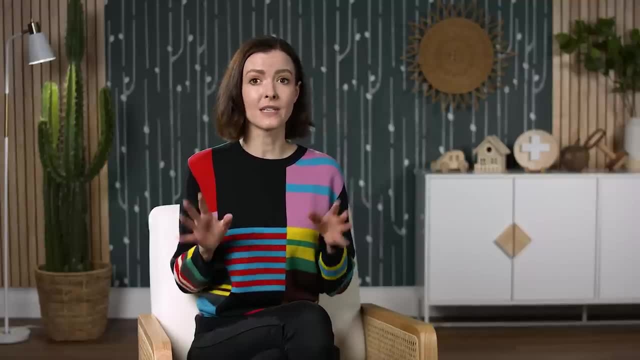 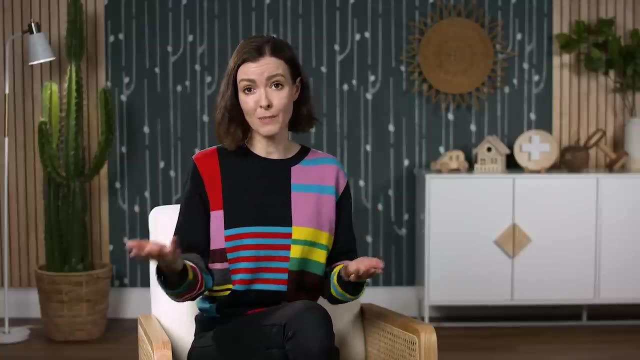 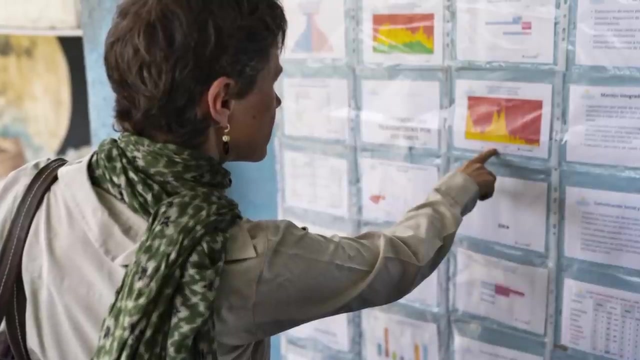 slice in common. Instead, enough component causes can combine in different ways to form a sufficient cause, And this enoughness varies from person to person. Now, disease models aren't completely human error proof. They're still invented by people and rely on data collected by people. 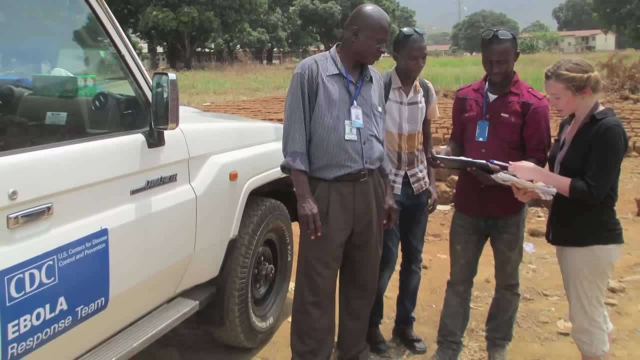 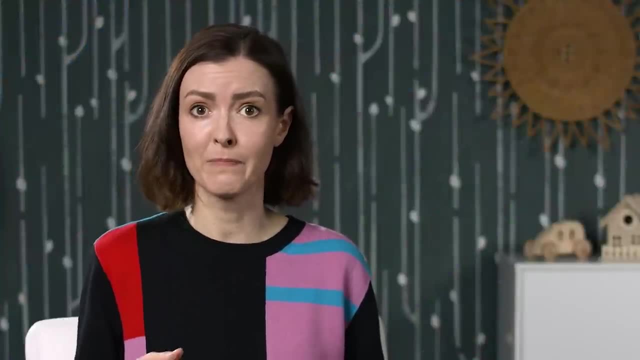 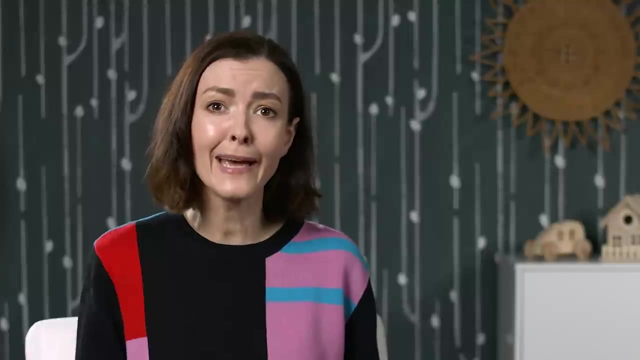 But the more data we collect and interpret, the better our health models get. And in a big, messy world where the causes of disease are often invisible, the cheese and murderous bedsheets go hand in hand. Epidemiology gives us the tools we need to make a little bit more sense of the world. 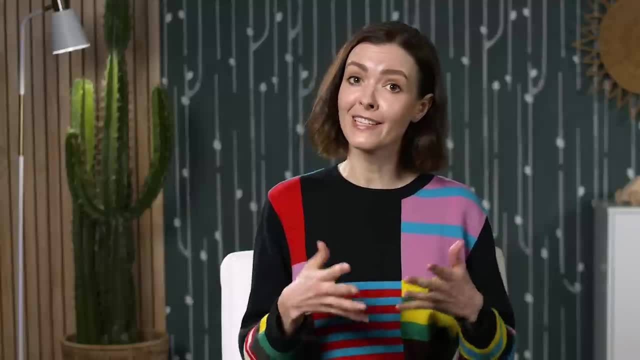 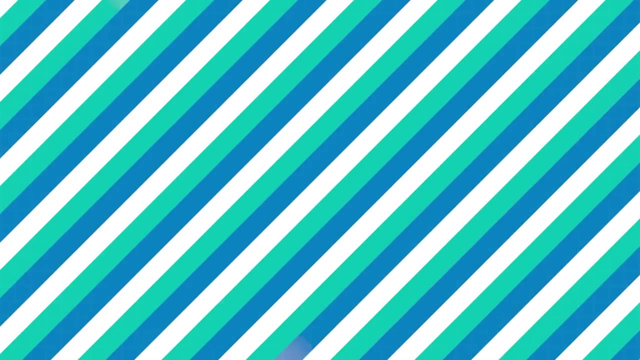 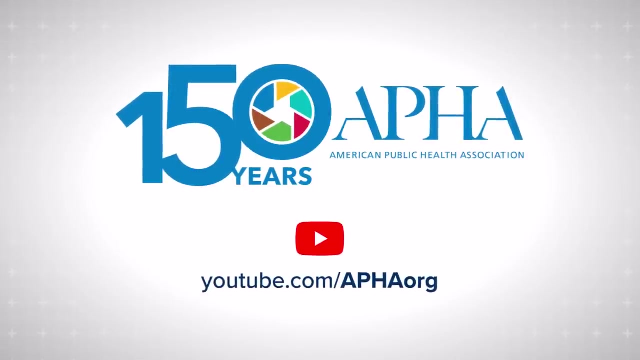 and how it impacts our health. We'll continue our examination of this big messy world next time when we talk about health systems. See you then. Thanks for watching this episode of Crash Course Public Health, which was produced by Complexly in partnership with the American Public Health Association. If you want to learn even more, 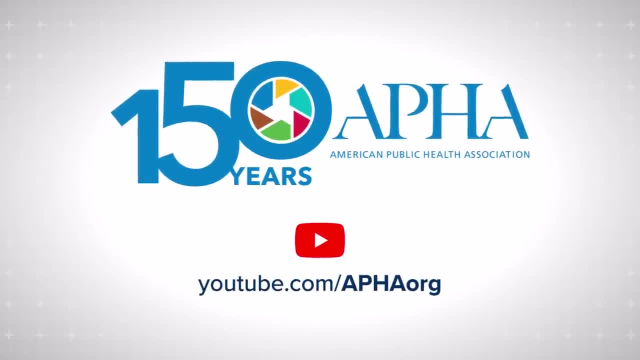 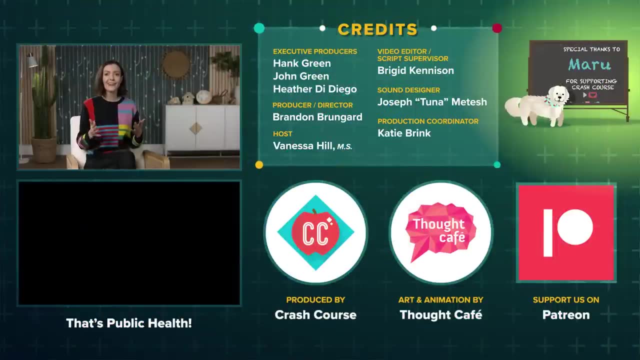 about public health. head over to APHA's YouTube channel to watch. That's Public Health, a series created by APHA and Complexly Crash Course was filmed in the Castle Geraghty studio in Indianapolis, Indiana, and made with the help of all of these smart people. 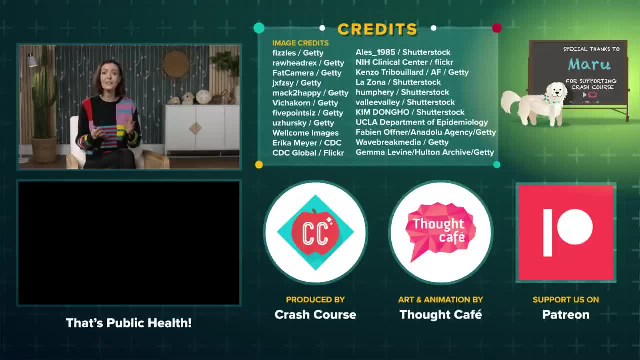 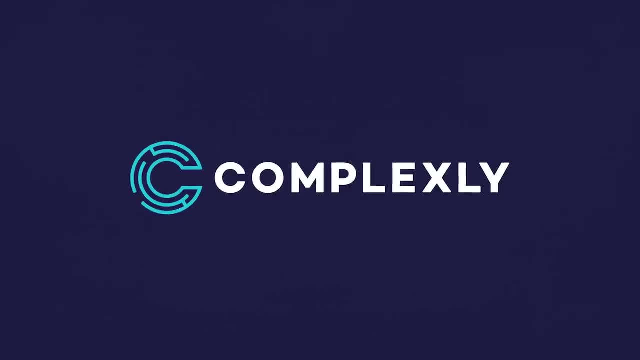 If you'd like to help keep Crash Course free for everyone forever, please consider joining our community of supporters on Patreon. To learn more about this series, visit our website at wwwpatreoncom.